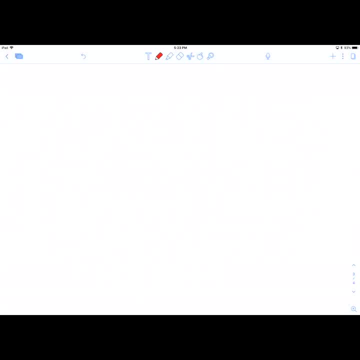 Just to wrap up our intro to graph theory, there are a couple of ideas that I want to mention real quick, Very simple things. again, A couple more definitions. First of all, when we talk about a graph, we can also talk about a subgraph. 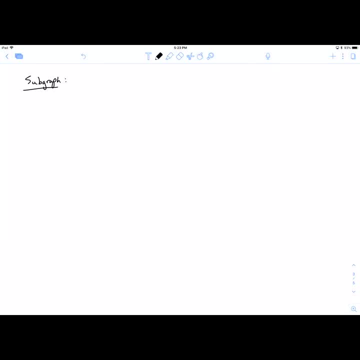 Kind of like when we talked about set theory we had subsets. A subgraph, you might imagine from the name, means a smaller graph that's sort of a piece of the larger graph. So to make a subgraph, say you've got a graph you're working with. 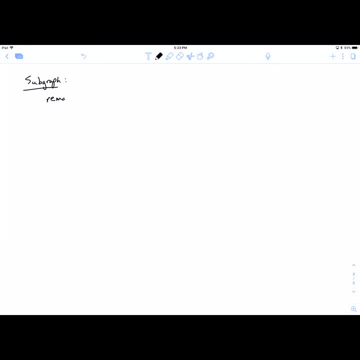 If you want to make a subgraph out of it, what you can do is remove some vertices, So one or more, And then, when you do this, you want your leftover graph right, the subgraph. you want that to still be a graph. 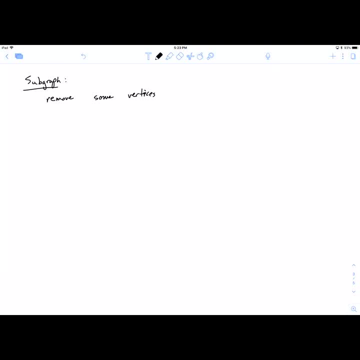 which means you can't. you can't have edges that go to nothing. So if you remove a vertex, you have to remove any edges that connect to it as well, so that you don't have these sort of orphan edges that go to nothing. 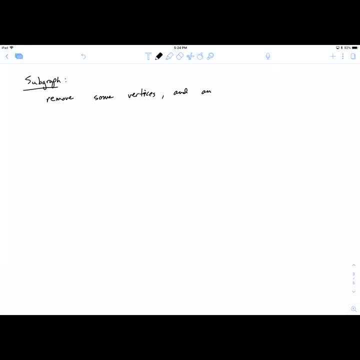 So remove vertices and then any edges that connect to a removed node. a removed vertex. So, for example, let's say we have a graph like this with nodes a, b, c, d and e and then connections edges, as shown. So to make a subgraph that's similar to what we did. we already have some edges and we're going to go ahead and add some edges to that. You want to use this as an example, So let's do a than a or five-STR. 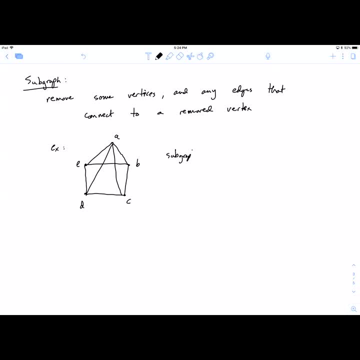 let's say, for example, the way we decide to make a subgraph is to remove the node D, to remove that edge there. so what I'm actually going to do to visualize this is I'm going to copy this over here and, rather than redrawing it, I'm just going 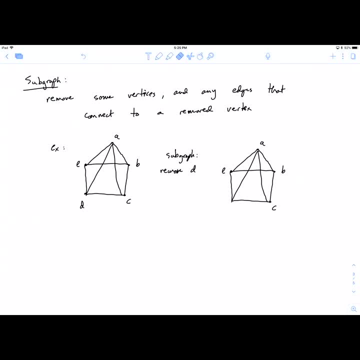 to erase. so if I erase node D, now we have three edges that connect to nothing. so if I remove those three edges, leaving this one behind, that would be an example of a subgraph of the first one. so a subgraph, the definition is just a graph. 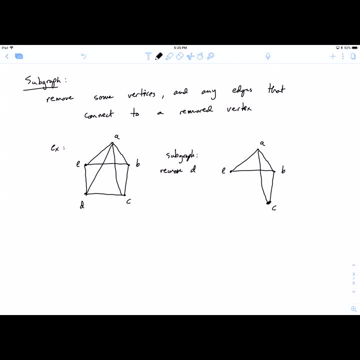 that is really a subset of another graph that has some of the nodes and some of the vertices and not any extra ones. so, for instance, if you had another edge like this, that would not be a subgraph of the first one because it contains an edge that the first one did not, so a subgraph. the idea is very. 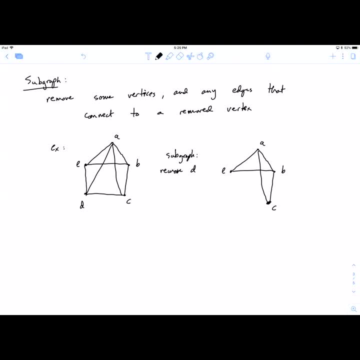 intuitive. it's just sort of a smaller graph contained within one, but it is significant that it's. it should be a graph itself, so it shouldn't have edges that go to nothing. another definition that we'll run across and we'll use here and there is the term degree. 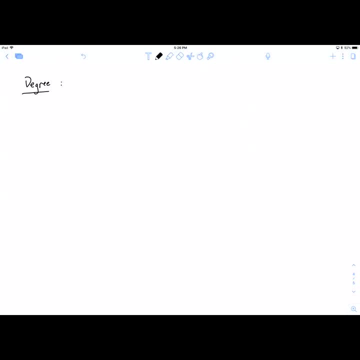 so we talk about the term degree. this is attached to a vertex, so we talk about the degree of a vertex. what you mean is the number of edges that connect to it. so for now, I'm going to talk about an undirected graph, and we'll come back to 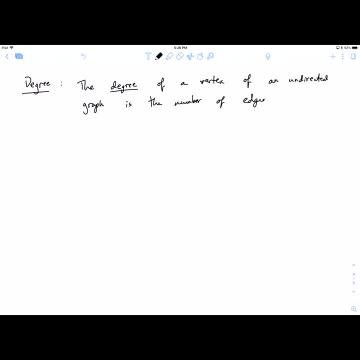 that idea in a second. so it's the number of edges that contain it. when I use the term contain it, what I mean is that connect to it. so I'm thinking about it from the sort of set theory idea of a graph where an edge contains two nodes if it. 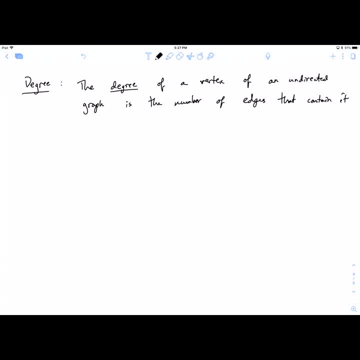 connects them, so the number of edges that contain it or the number of edges that connect to it. so, for example, let me draw the graph here: a and b, c, d and e and let's draw connections between them. notice, by the way, this is not a simple graph. we have both loops and multiple. 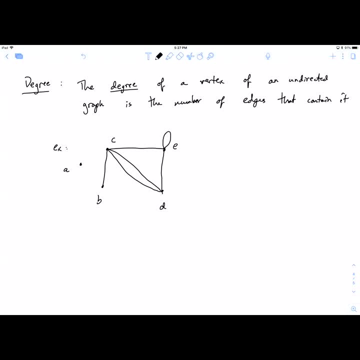 edges. so that's a multi-graph. we can go through this graph and we can see that there are no edges that connect to it. so we're going to go through and kind of count the degree of each vertex just by looking at how many edges connect to it. so I'll put the 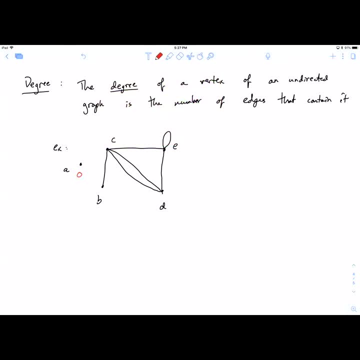 degree in red. the degree of a is obviously zero because there are no edges that connect to it. it's an isolated node, so it has no degree. b would have a degree of one. c would have a degree of four, right, because there are four edges coming into it. 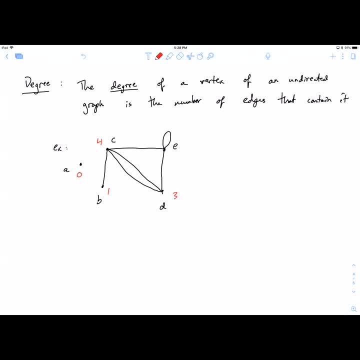 D would have a degree of 3, and then we get to E, and E is interesting because you might look at it and you might say: well, there are three edges that connect to it, because this edge is really only one and so it connects to it just once, so you might count three. 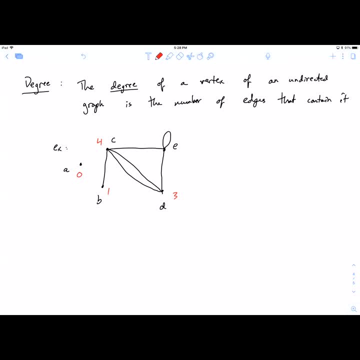 But it turns out by convention we count a loop twice, and so really what you're doing is you're looking at this node and looking at how many edges come into it or go out from it, And there are really four of those, even though two of them belong to the same edge. so you 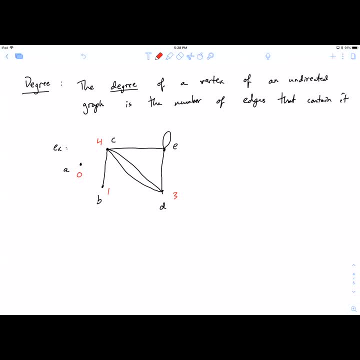 count a loop twice And the reason for that. we'll talk about one example of why that's important in a second, when we talk about some conclusions. we can draw about degrees, but for now just recognize that a loop counts twice. So I mentioned that this. 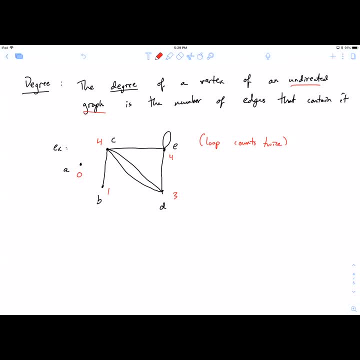 definition belongs to undirected graphs. With directed graphs you can still talk about degree, but more likely you would talk about the outgoing degree and the ingoing degree, So each vertex would have two degrees associated with it. how many edges go out of it? and 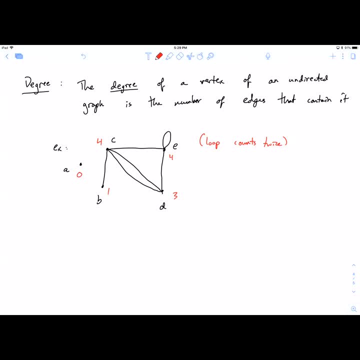 how many edges come into it, and you would count them just like you do here. So degree: this concept also applies to directed graphs, but you just need to account for the possibility that you have an incoming degree and an outgoing degree. There are two simple theorems we'll look at that will relate to degree, and both of them. 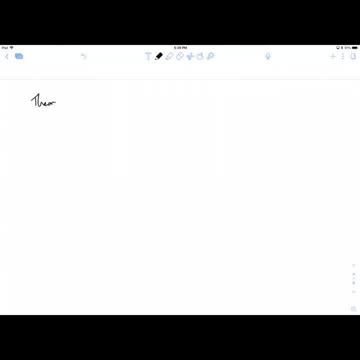 should be fairly straightforward to understand. So, first of all, one theorem says that if you add up the degrees for all the vertices, again in an undirected graph, you can think about how you would change this for a directed graph. but for an undirected graph, if you add up all the degrees for all the different vertices. 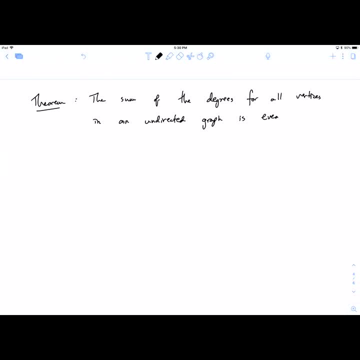 what you will get is an even number. now let's go back and look at our example. if we add up the degrees, we have 1 plus 4 plus 4 plus 3, which is 12. sure enough, that's even. and you can keep drawing examples and trying to to look at. 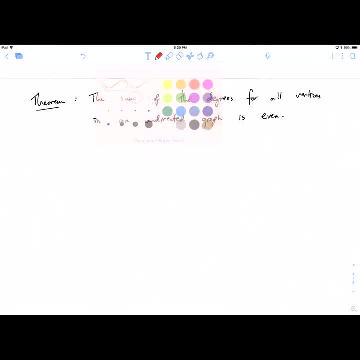 this, but the proof for this- and I'll put proof here in quote marks because we're not going to write down a formal proof- but the proof is really pretty simple. it's pretty easy to understand. if you think about this, maybe you want to stop the video and think about it for a second and 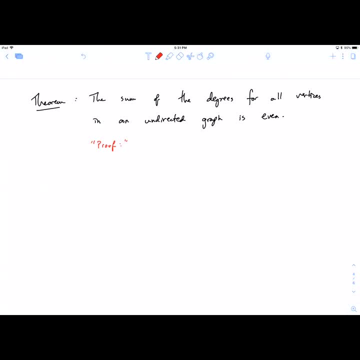 think about how you would explain or prove or verify that this is true. but the reason this is true is that, if you think about it, each edge that you draw contributes 2 to the total number of degrees. in other words, take this edge, for instance, when I draw that edge. 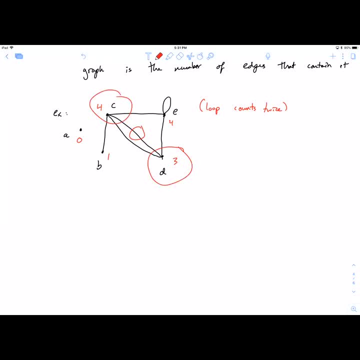 it's going to add 1 to the degree of D and 1 to the degree of C, and so each edge contributes 2 to the total sum. so if you add up all the degrees, it's however many edges you have times 2, that's. 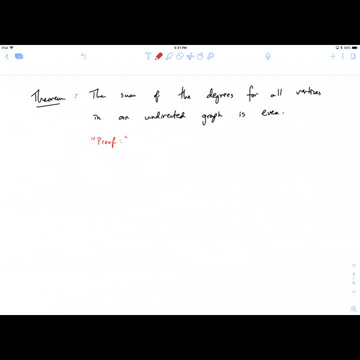 all it is. so it's guaranteed to be, even because you have an integer number of edges. so very simple proof, just this idea that each edge contributes 2 to the total number of degrees in the graph. now this leads us into a second theorem. we can use that first one to prove this one. this: 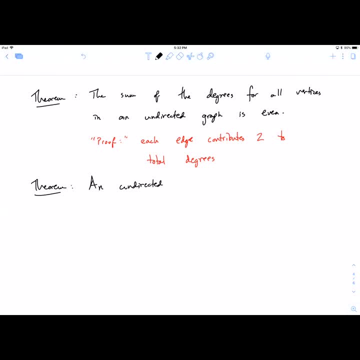 theorem says that if we start with an undirected graph again, if you change the graph to a directed graph, I'll let you think about how this would change. undirected graph has an even number of vertices with odd degree. in other words, if you go through and do as we, 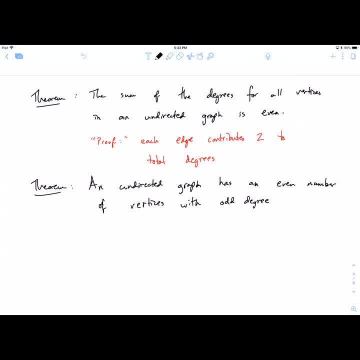 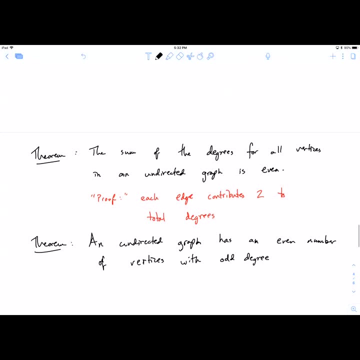 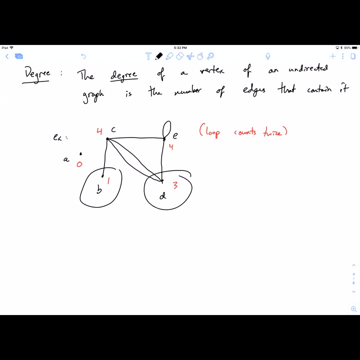 did, counting the degree of each vertex. if you look at the ones that have an odd degree with them and you count those up, there's going to be an even number of them. in our example, if you go through and look for which ones have an odd degree, you find two of them. so there's either going to be. 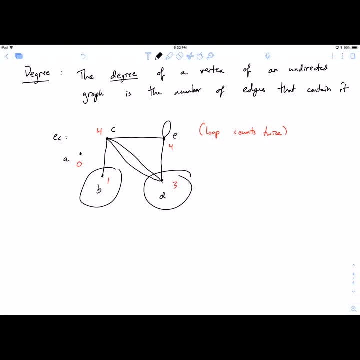 no nodes with an odd degree, or two of them, or four of them, or six of them, or eight of them, but you'll never have a graph drawn correctly that'll have three nodes with odd degree. now let's think about why that's true. again, you might want to pause and think about how you would prove. 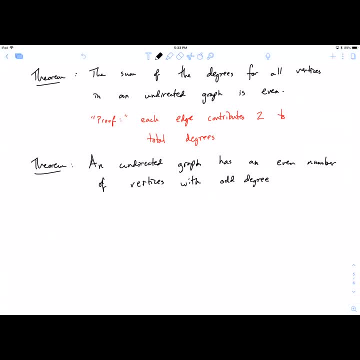 this. it's a little bit more involved than the last one, but we can use the last one to prove this. so, to start out, we'll use the last theorem, which is that if you add up all the degrees in your entire graph, you get an even number, and 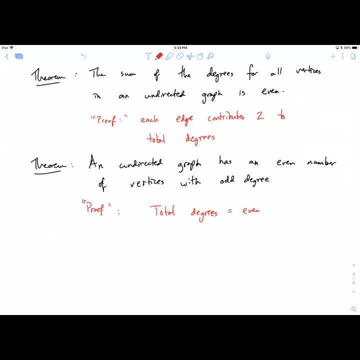 then we'll think about if that's true. we can split this up and think about the degrees that we get and from even nodes, and we can think about the degrees from odd nodes, and so if we add them up separately, so i'll use- we've used this summation notation before, so this just means add up all the degrees. 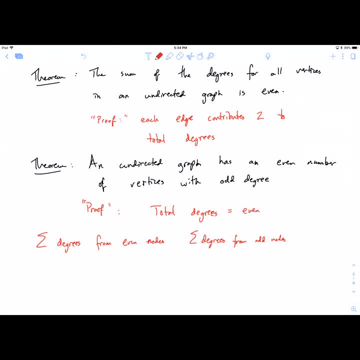 from each of them. you add up all the degrees from the even ones and all the degrees from the odd ones and then, as those together, you've got all of your degrees from the odd ones and then you've got your degrees. so this total degrees you can split into these two categories where you think about. 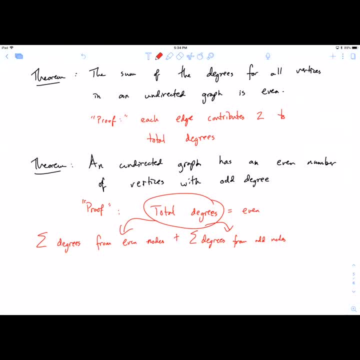 separating out your even ones from your odd ones and then adding them up separately and getting two different sums. if you do that, that still needs to be even right, because the total degrees all have to even ones. now, if you think about this, this first part- the degrees from the even nodes- is 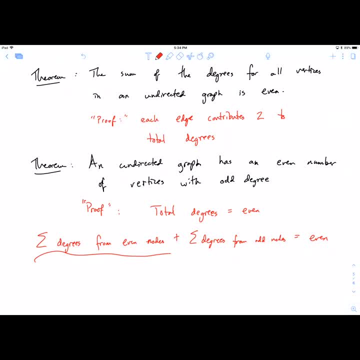 definitely going to be even right, because if you start with an even number of nodes and start adding them up, you're going to get to an even value. so the degrees from odd nodes have to be even as well. so for the first one, if you add even numbers together, you get an even number. so 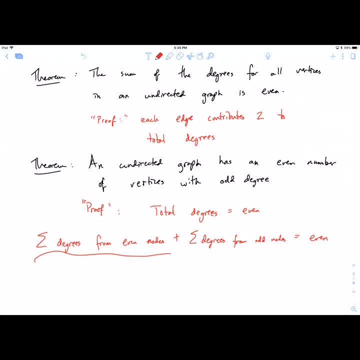 if you've got an even number of of nodes- or all the nodes that are that have an even degree rather- and you start adding those up, you're going to get even numbers every time you add one on. so no matter how many even nodes you have, you're going to get an even number from that. 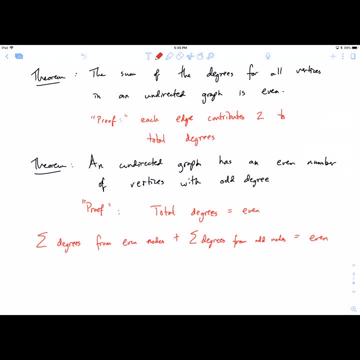 so if you're going to add these two together, back when we were talking about proofs, we looked at things like this and it turns out that to get an even number here, if this is even, this also has to be even right, because the sum of two even numbers is even. the sum of two odd numbers is even. but 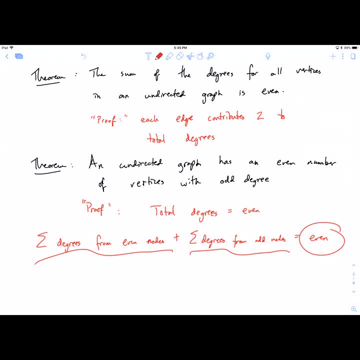 the sum of an even and an odd is odd. so if the first one is even, the second one has to be even. so, if these odd nodes, we add them up with a little bit of thought, you should be able to see why this. there must be an even number of these. 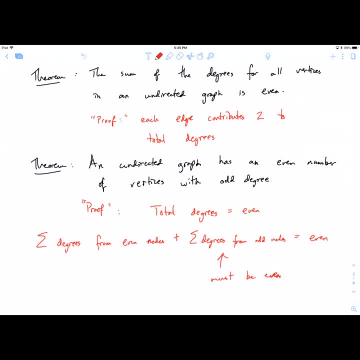 because again, if you add two odd numbers together, you get an even number. but then if you add on a third odd number, you get an odd number. adding a fourth odd number goes back to even, and so if this has to end up being even, there must be an even number of them that you add up. so if you're going 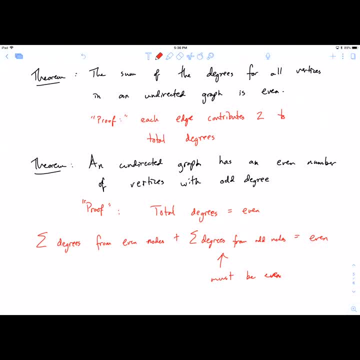 to get an even number of these. you're going to get an even number of these, so, anyway, you can think about that a little more on your own, but it's a relatively simple proof just using the previous theorem. but things like this are the kind of things that Euler started thinking through when 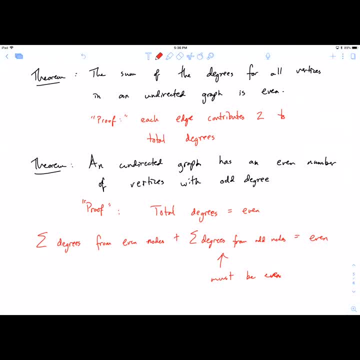 he started developing graph theory and kind of looking at what implications follow from just the